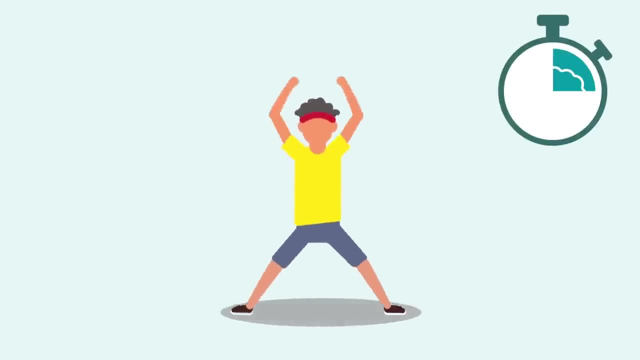 about them. Physical activity releases feel-good hormones called endorphins, which help us sleep and feel better. It also improves our physical fitness, which tends to make people feel better in general. Even small amounts of regular physical activity can improve your mental well-being. especially if it's doing something you enjoy. Physical activity is even a recommended treatment for some types of depression. You can get active at your own pace, in your own way. There's no need to join a gym or even spend any money. Simple, small changes in our day-to-day. 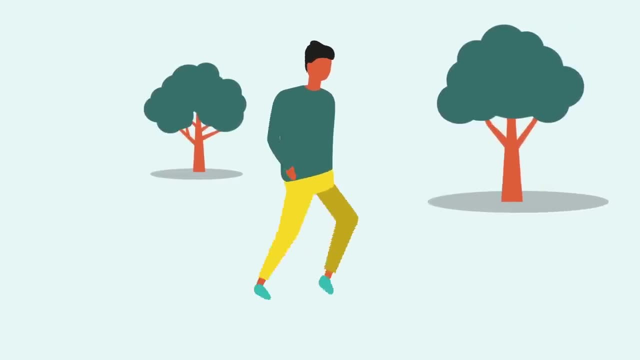 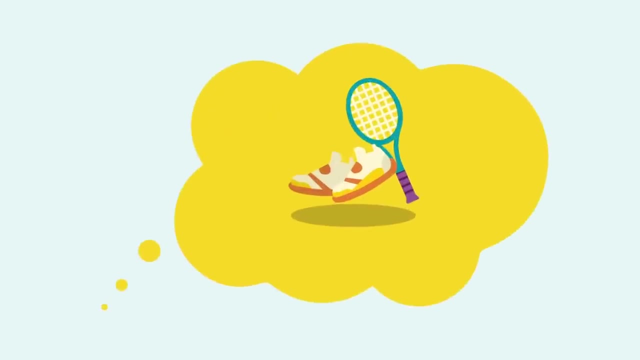 can make all the difference. Taking a brisk walk at lunchtime or walking to get where we're going, getting active in the garden or cycling once or twice a week are great options. If there's a type of activity you used to enjoy, think about how you could pick. 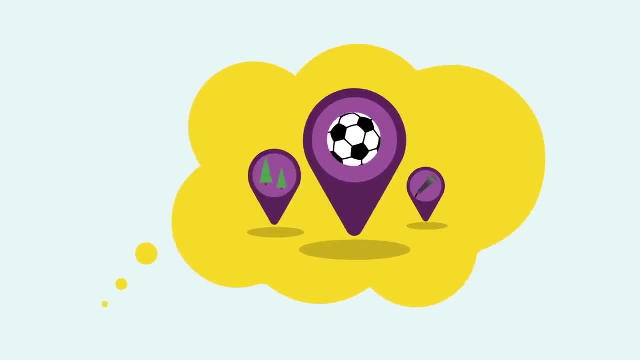 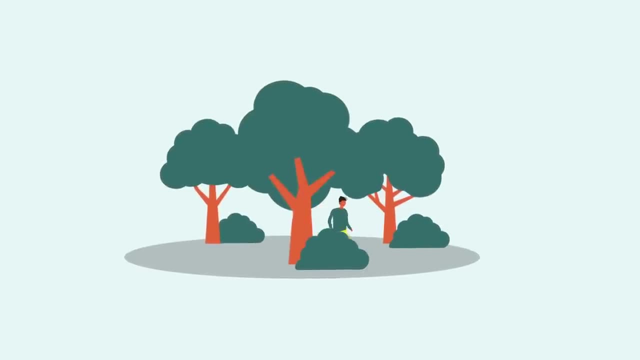 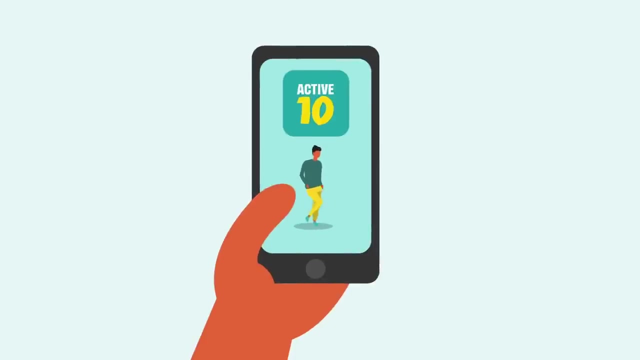 it up again. For example, there are lots of local groups and sports teams open to all levels of ability. What's more, studies show that time in green spaces is beneficial. So head to your local park if you can. If you need a little help fitting more physical activity into your day, try the. 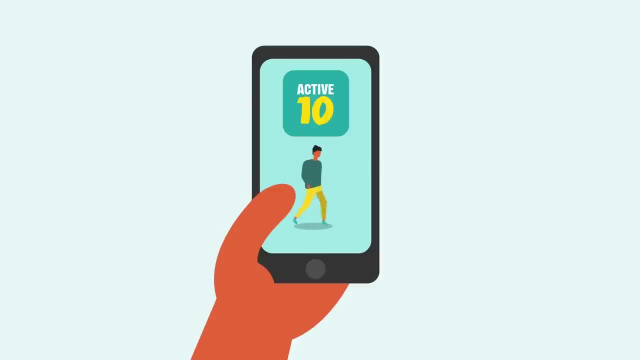 Active 10 app. It helps you get short bursts of brisk walking into your day. There's also the fantastic Couch2Five app. It's a great way to take a break from your day-to-day activities. and take a break from your day-to-day activities. There's also the Couch2Five app, which will get 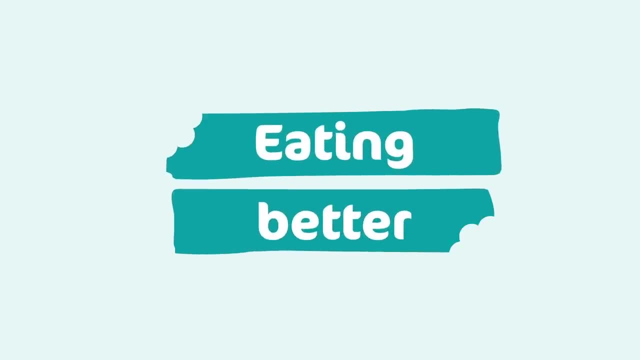 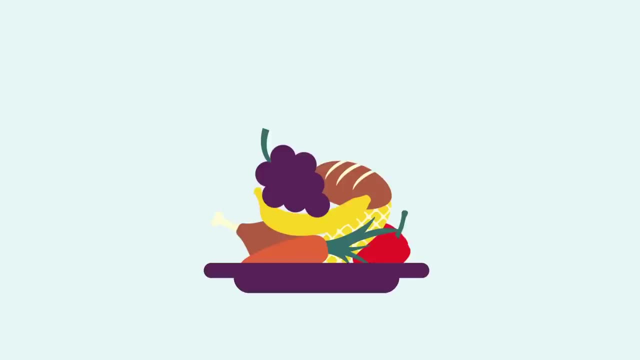 you up and running in just nine weeks. Eating better can play a big role in our health and well-being. It won't come as a surprise to learn that what we eat, and how much, plays a big part in our physical health, which can impact our mental health too. Ideally, we should aim to eat a. 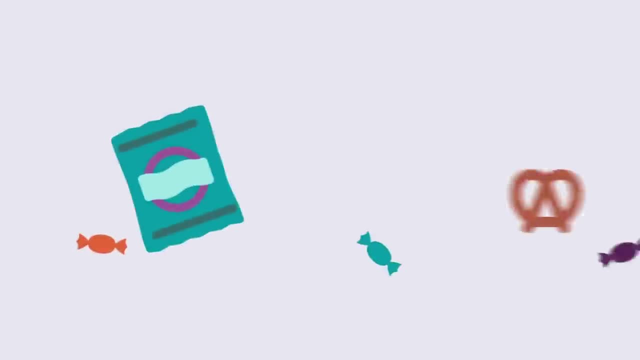 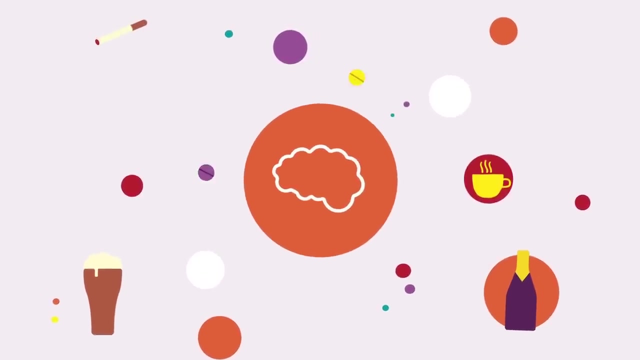 healthy, balanced diet with plenty of fruit and veg. It's important to keep an eye on your calories and minimize foods that are high in sugar, fat and salt. For helpful tips on eating a better diet, check out the One You website. Alcohol, caffeine, tobacco and even drugs may seem tempting when we're stressed or tired. And when we use them to try and cope. the idea of stopping them can feel like it would make things even harder, But they can cause more problems than they solve, especially long term. All these habits can complicate our sleep patterns and affect how anxious and depressed we feel. 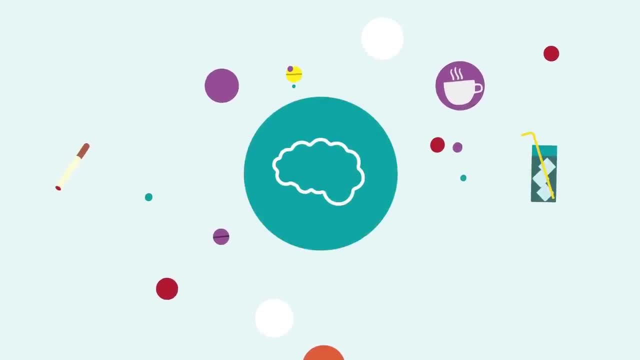 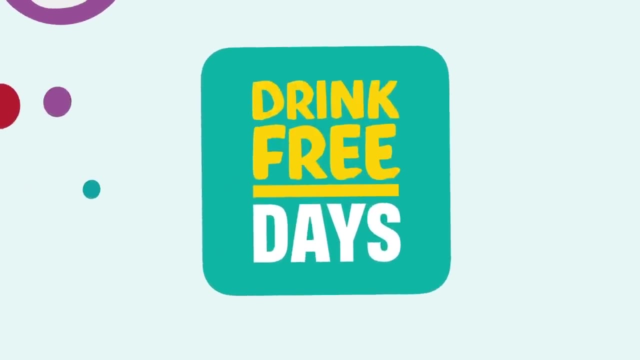 So try cutting down or even quitting, and remember that there's support available. Alcohol in particular can worsen our moods, so cutting down can really help us feel better. For more help cutting down, you can download the Drink Free Days app. 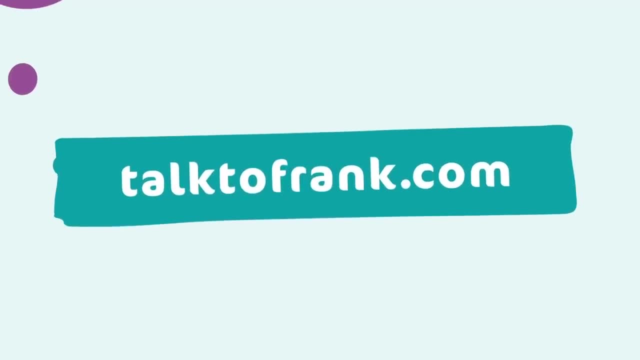 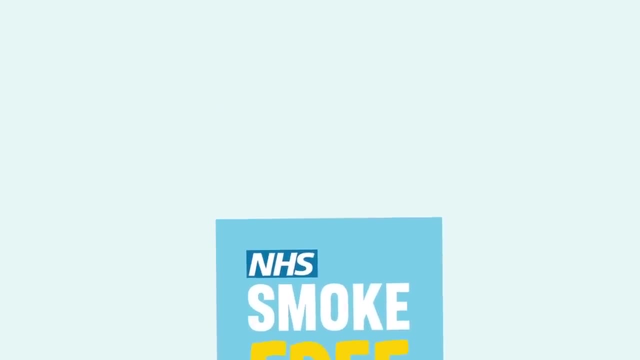 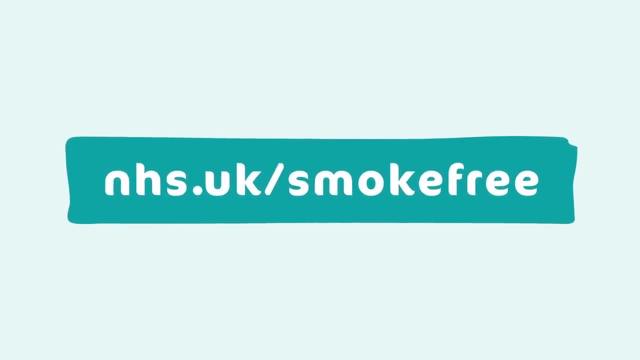 And for help cutting back on drugs, visit the Talk to Frank website. As for cigarettes, stopping smoking is one of the best things you can do for your body and your brain. You'll breathe easier, feel better and save money. Check out nhsuk smokefree for advice and support. 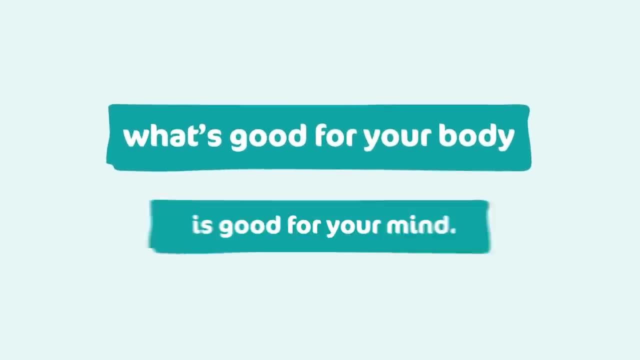 on quitting Whatever you choose to do. what's good for your body is good for your mind. 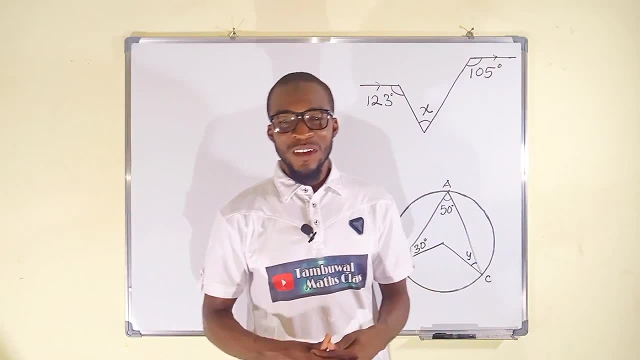 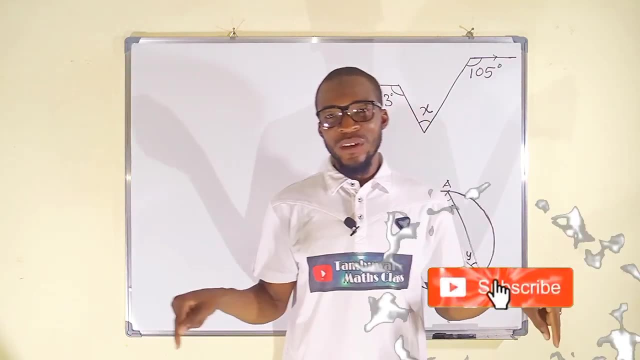 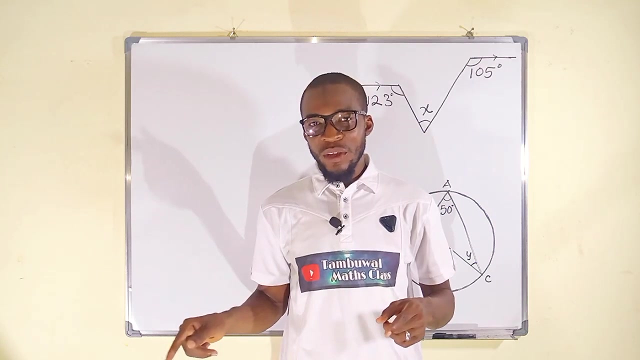 Hello, good morning viewers. In this tutorial we are going to find a solution to these two geometry questions. So if you are new here, consider subscribing. Press the bell icon so that you will be notified whenever I upload a new content, And don't forget to share to your. 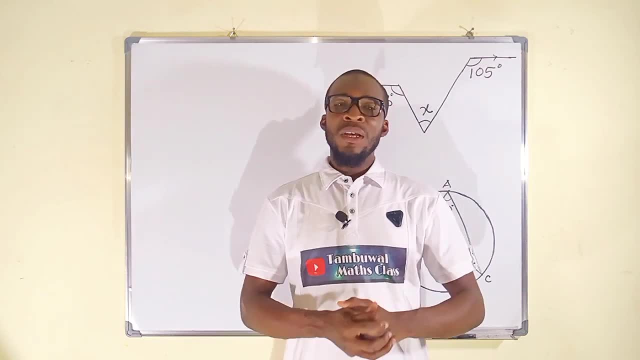 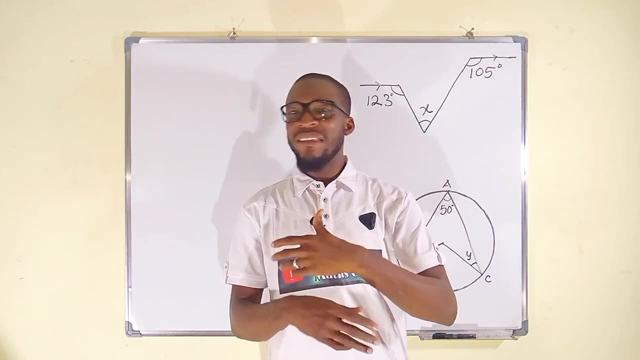 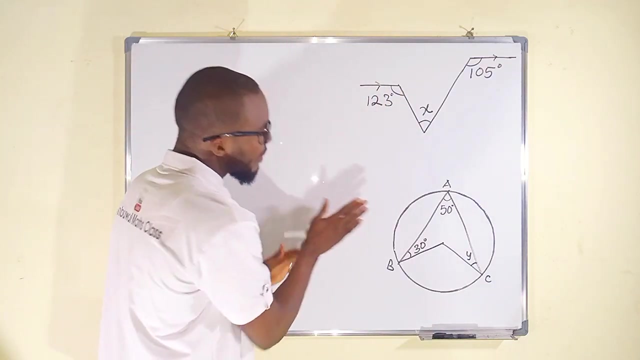 learning colleagues, Don't forget also to hit the like button. One interesting thing about geometry: the way I will solve these problems might be entirely different from the way you will solve it. So now let us give this a try. We have two problems here. Let us start with this one. 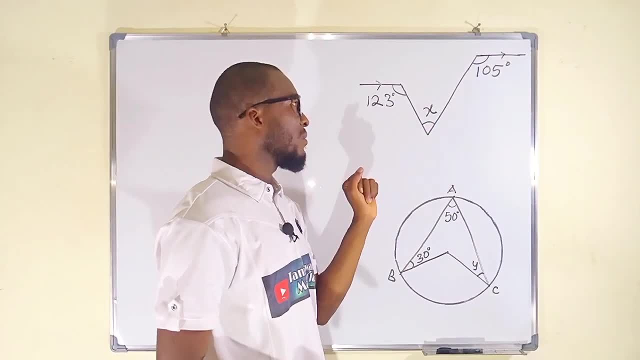 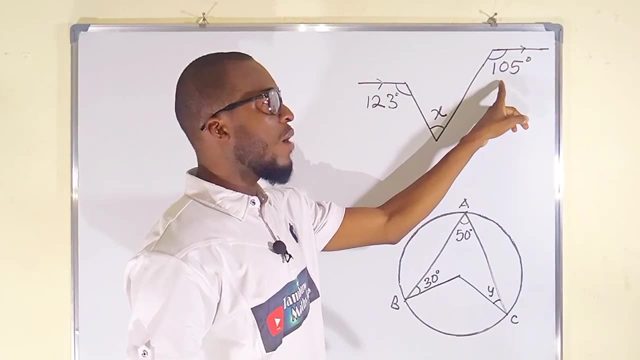 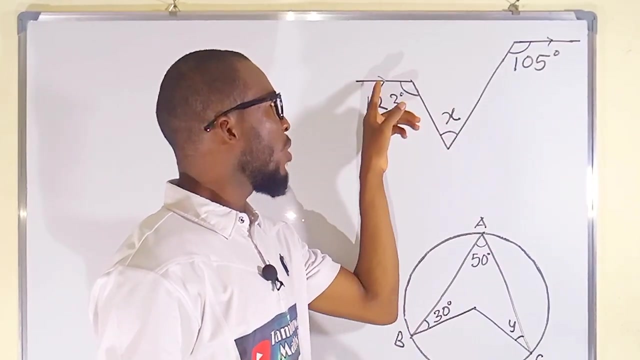 We want to find this angle, which is represented by x. But let us observe the diagram carefully. We have 123 degrees here and we have 105 degrees here. But of that, these two lines, they are parallel to each other. This is why we have these two marks indicating that no matter. 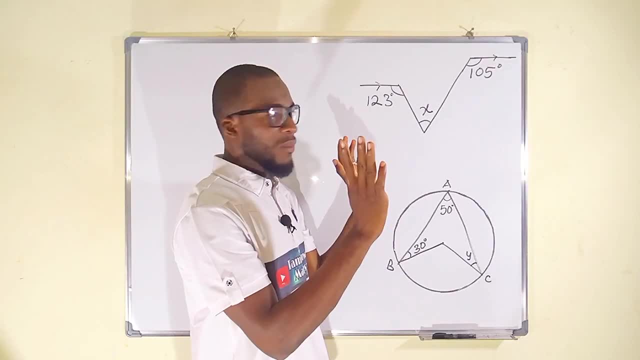 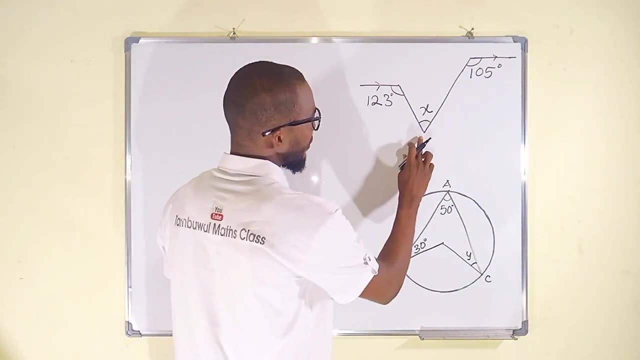 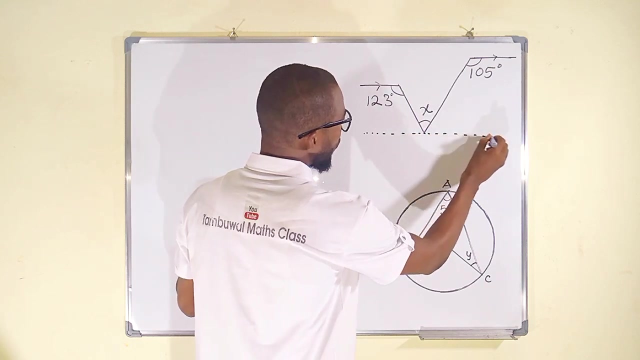 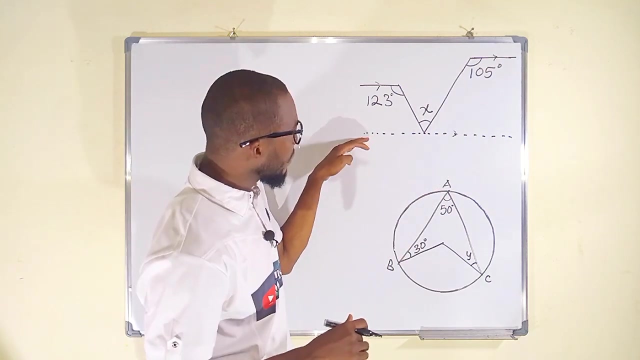 where they get to. they will never meet. So therefore they are parallel. So now we can construct an imaginary parallel line just beneath this angle, So such that it will be parallel to the two lines this and this. So this should also have a mark here. What does this mean? It means that 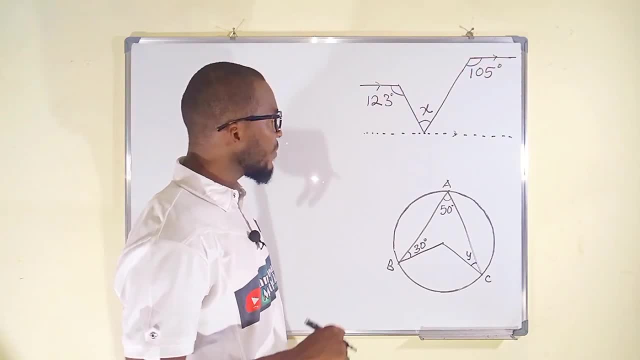 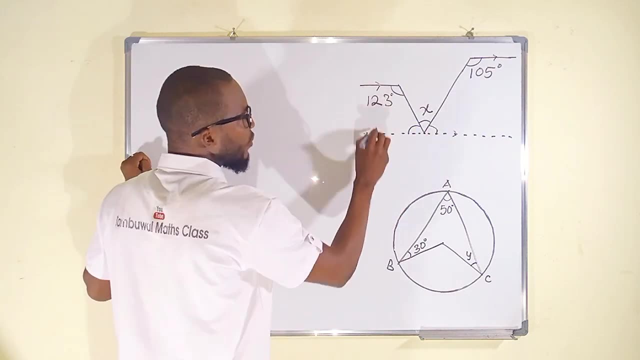 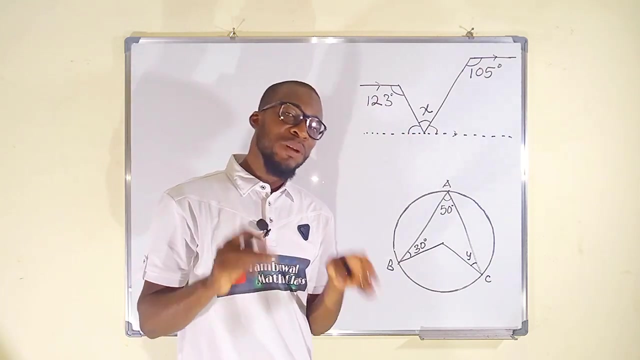 this line is also parallel to these two lines. All right, let us observe this: This angle here and this other one. Remember, if these two lines are parallel to each other, this angle and this angle are said to be supplementary. If they are supplementary,